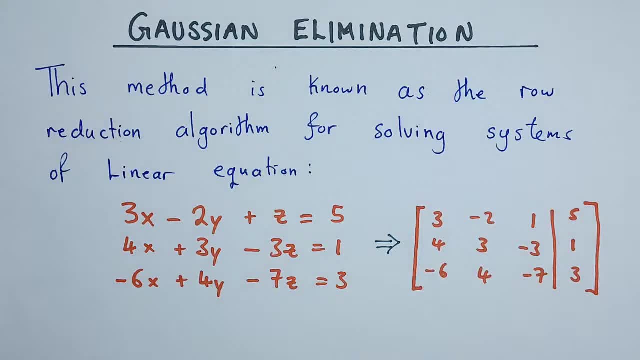 you put a zero instead, Don't just leave it blank. So it means that there'll be a zero there. So the way to achieve here is to make sure that these three values become zeros. So these three values must become zeros, And then these three values here must become ones. So we need zeros here and 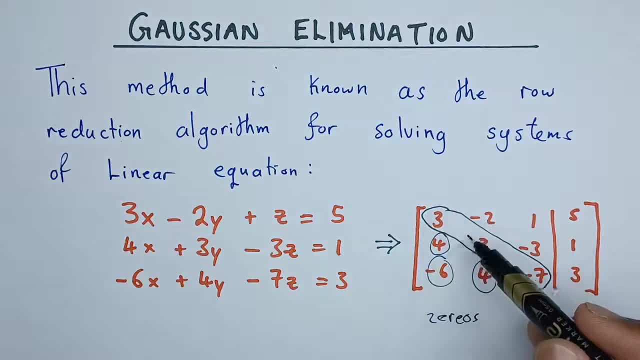 we need ones in that major diagonal And of course we shall do that by the row operation. like we said, You will see how it's easy to use the Gaussian elimination. So also understand that whenever you are playing the Gaussian elimination, it's if you want, you can leave it in this simplified form. 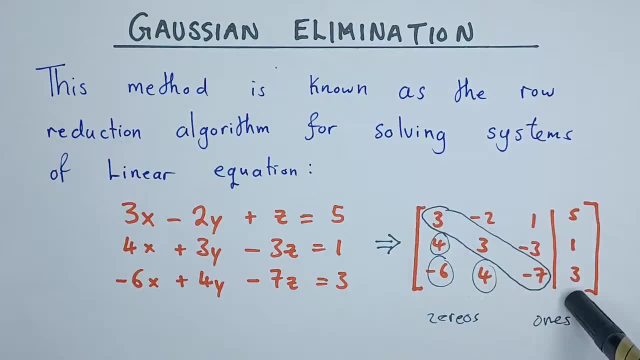 where you put zeros everywhere, then just ones here, then you get your answers direct. But it's just easier to have zeros here and ones in the major diagonal. Okay, so I'll give you an example. then I'll come back to this particular example after the one that we shall do. So let's jump. 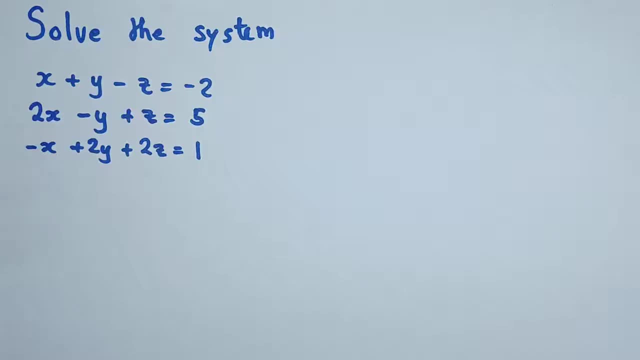 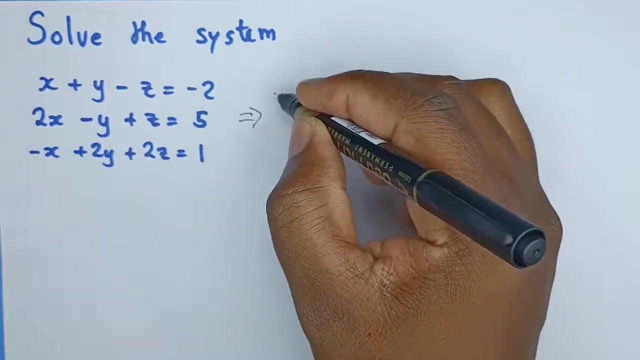 and look at how to apply this method. Okay, so we have this, these three equations. then we want to apply the method of Gaussian elimination to solve. So to start with, like I said, let's put them in matrix form. So this will be: we'll have one, two negative one, We're getting the coefficients for. 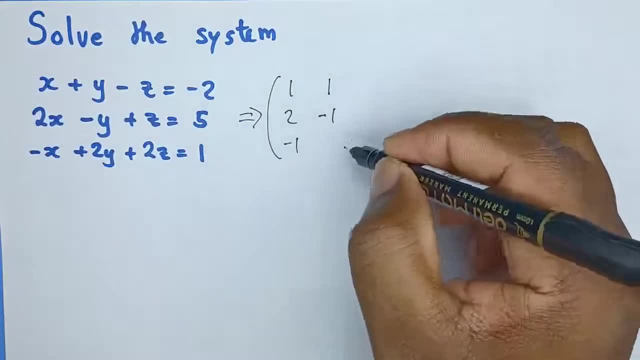 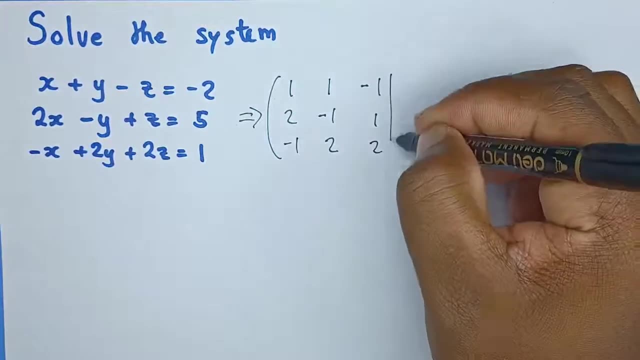 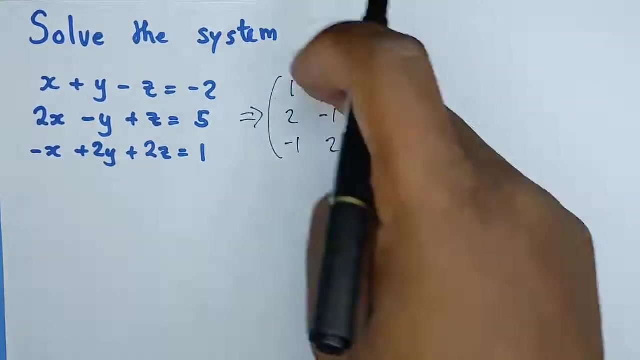 x. The coefficients for y: we have one, negative, one and two. The coefficients for z: we have negative one, one and two. Then we write down these values on this side, which is like that. Okay, so now remember, we need ones in the major diagonal and we need zeros here. So let's apply. 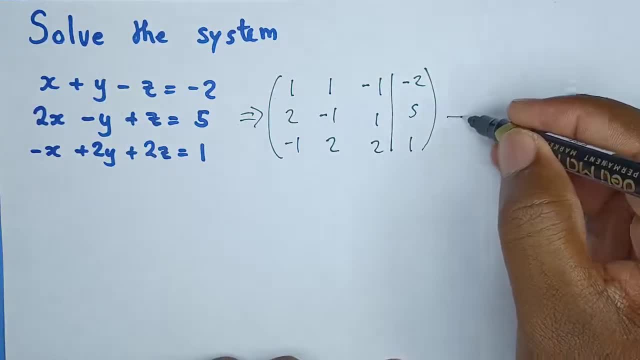 some row operations. Okay. so in our first row we're okay because we have the one here, but here we need a zero. So, since we need a zero, what we're going to do is we're going to multiply one by two, multiply row one by two, then we subtract row two, so that whatever we do here- yeah, this will just. 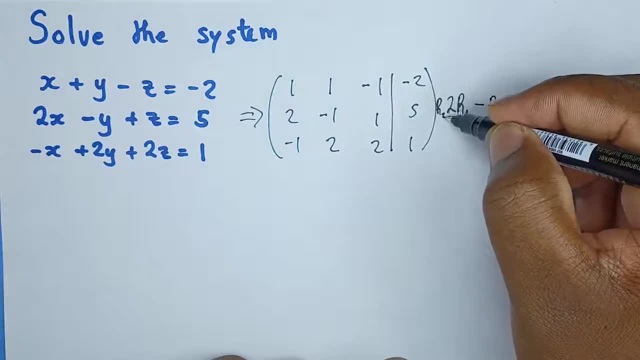 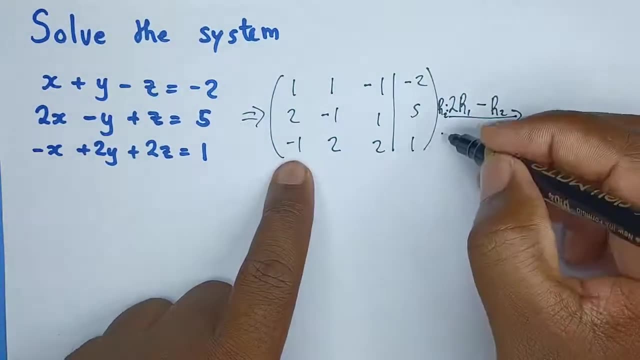 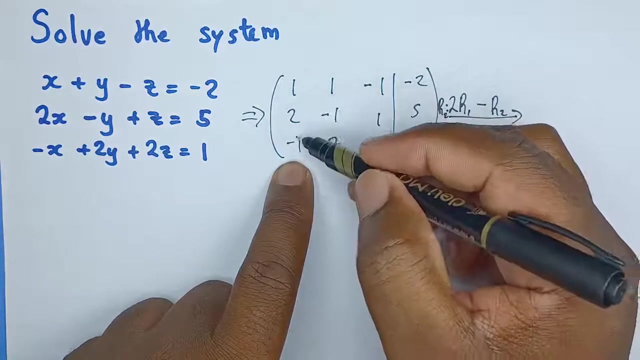 give us a zero. Now, remember, this is being applied on row two. I'll try it there like that. Then for the next one, again we need a zero here. So we're going to say the operation is on row three. We're going to add 1 and negative 1, because if we add these two we get a zero here. So the operation. 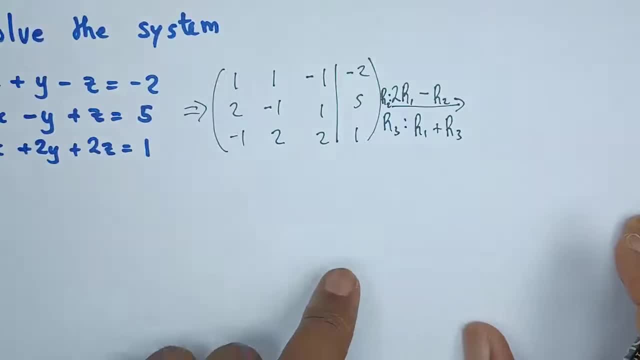 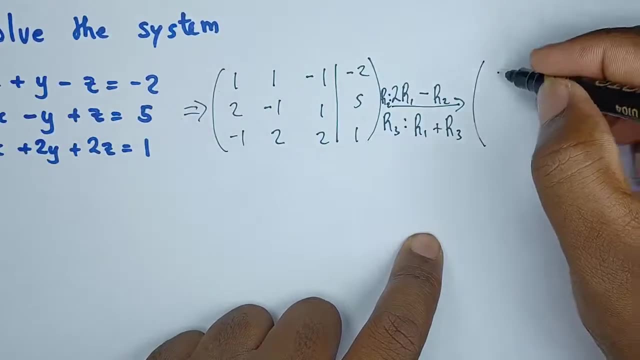 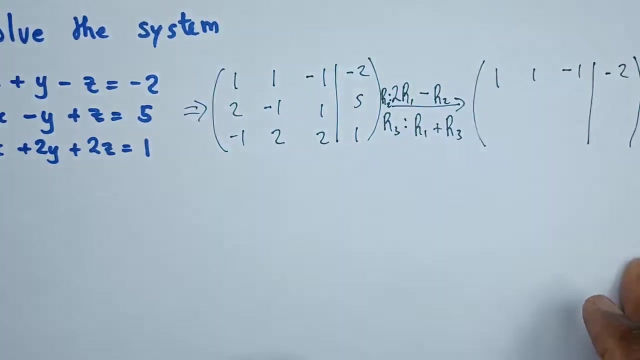 now, if you look at what I've done here, you can clearly see that I have not applied an operation for row 1, so row 1 will remain as it is. so row 1 is 1, 1 negative, 1, negative, 2 like that. then the only operation I'm going to apply here: 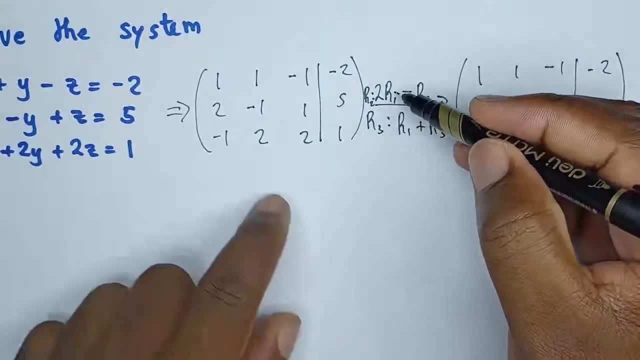 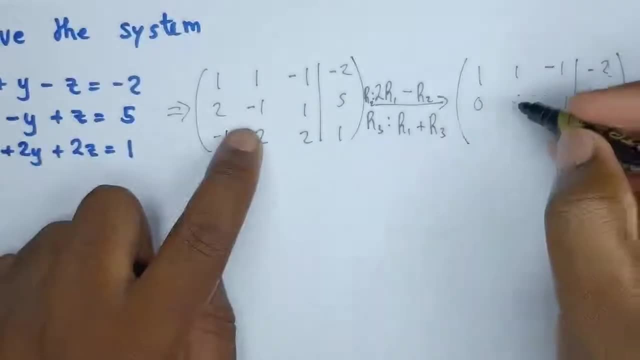 will be on row 2. so 2 times row 1 will get a 0 here. 2 times row 1, that will be a 2 minus this one will get a 3, or they'll add 2. that will be negative: 2 minus 1. 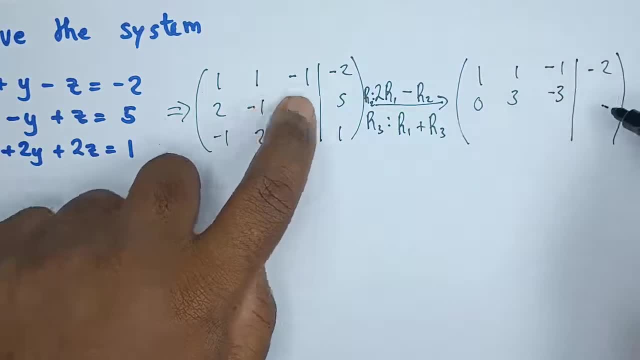 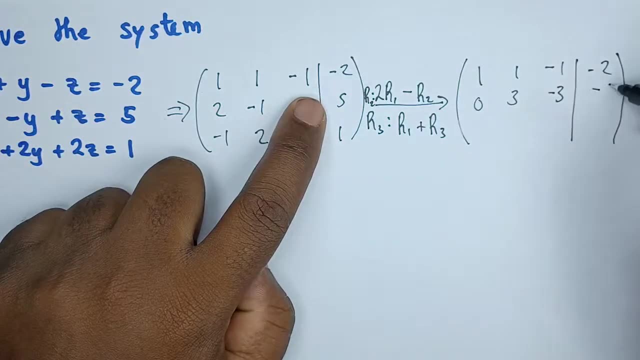 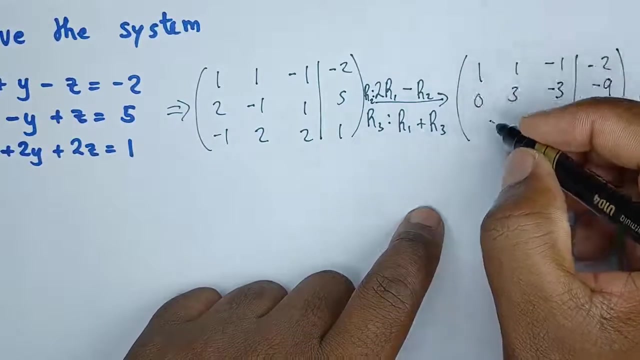 will get a negative 3. 2 times negative 2 is negative 4. negative 4 minus 5 will get a negative 9. so I've applied in row 2, let's apply in row 3. so in row 3 we're just adding everything. so to start with, add row 1 and row 2. 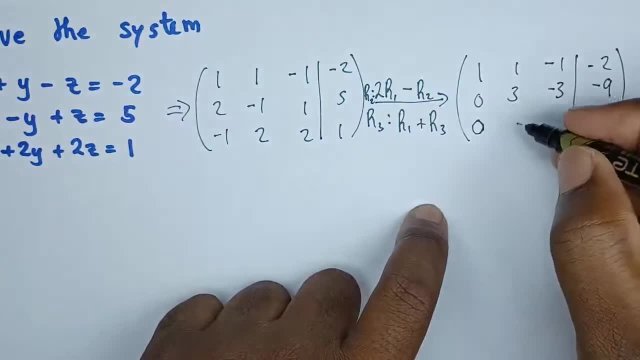 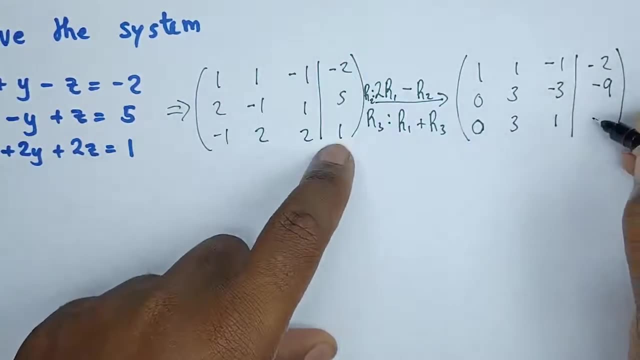 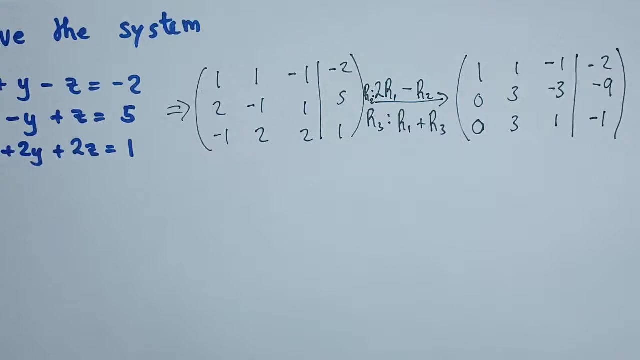 get a zero. here we add row 1 and row 2, sorry, row 1 and row 3. rather will get a 3. here we add these two, get a 1. add those two and get negative 1. okay, so if you look very carefully, what we have achieved so far is obtaining a 0 here. 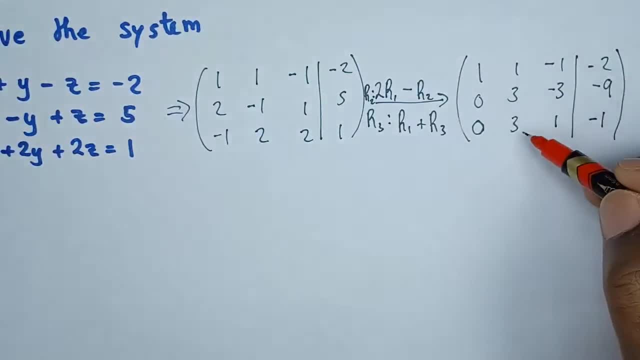 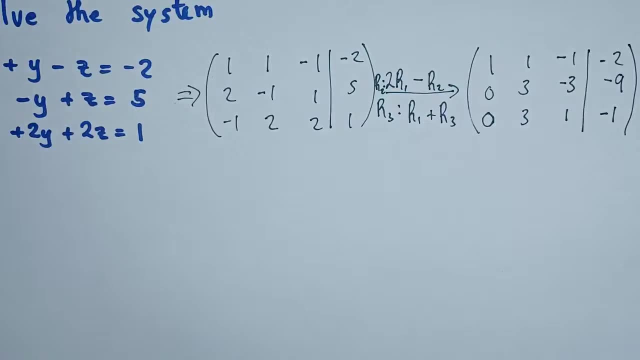 and 0 here as well. so the only thing we need now is a 0 here and the 1 there. then we are set. so the first operation I'm going to carry out will be in row 3. so I'm going to add원 1 and row 2 right here, because it is nothing but a 1. so the only thing we need now is a 0 here and the one there. then we are set. so the first operation we will carry out will be in. 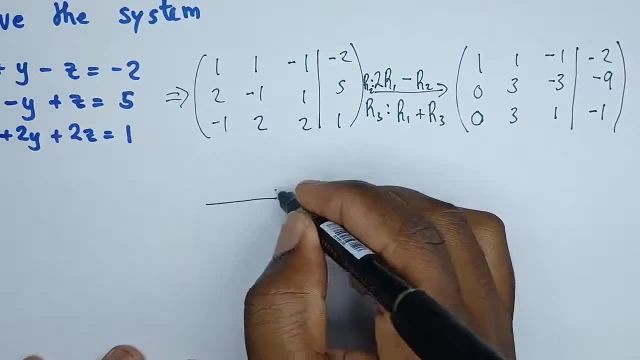 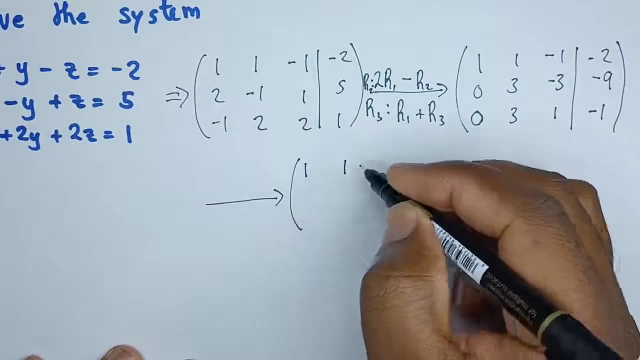 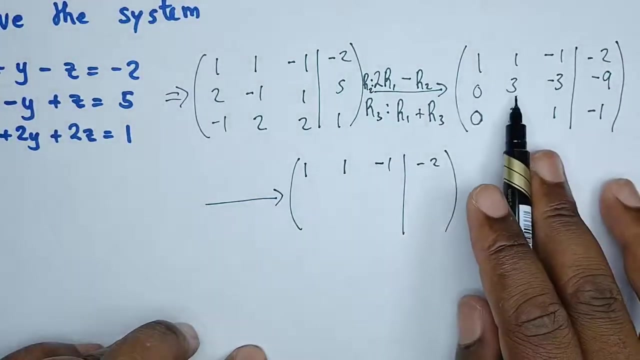 So the first operation we will carry out would be in row two. remember row one is already set, so in row two let's write row one as it is. so one is one, one, one negative, two, like that row two, the operation we're going to carry out. remember we need a one. 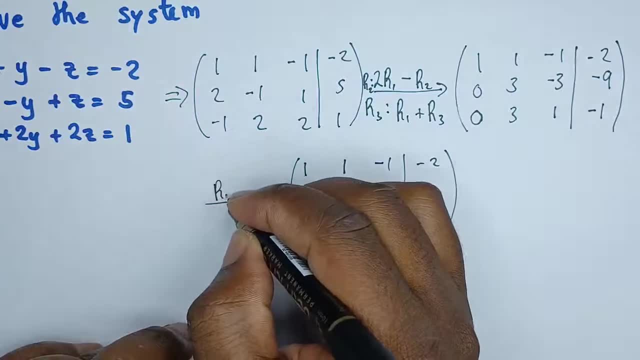 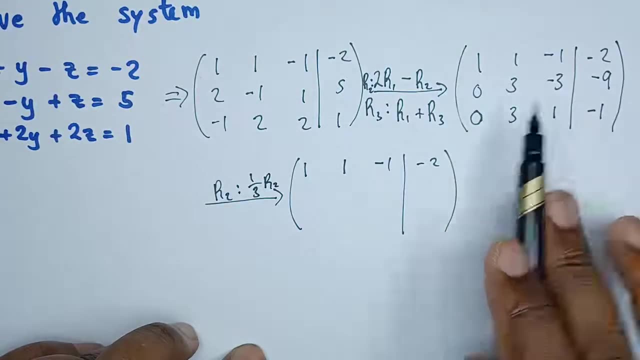 here. so let's divide everything in row two by three, like that. so divide everything in row two by three, or multiply it by one over three. so zero times one over three is zero. three times one over three is one negative. three times one over three is negative. one nine over three, you'll get a. 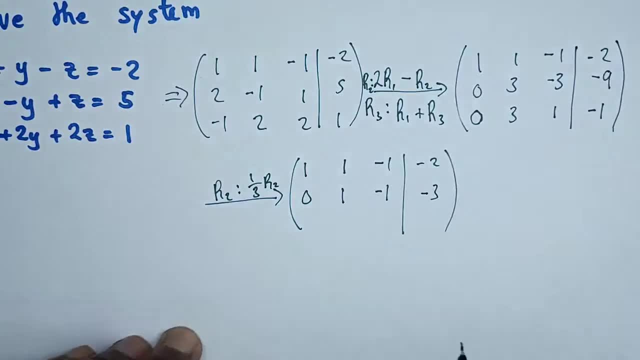 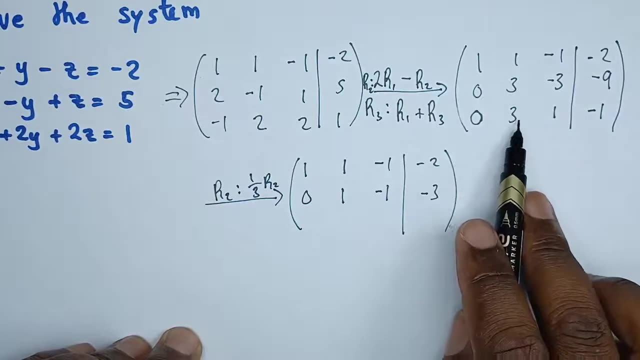 negative three, because the nine is a negative. okay, when we look at row three, we need a zero here. so to get a zero here we can subtract these two three minus three. we just give us a zero here. so the operation in row three will be row two minus row. 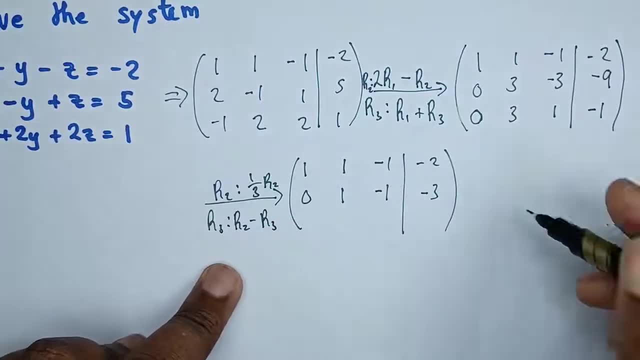 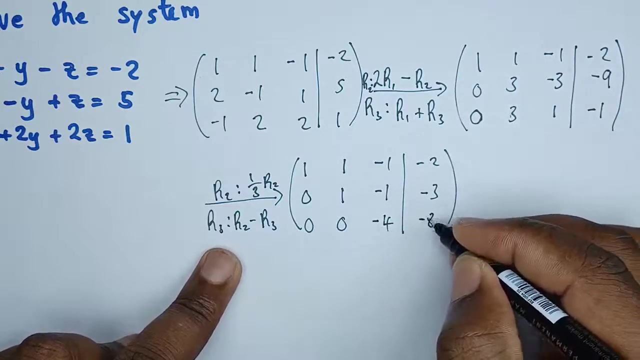 three. if you want, you can say: row three minus row two is just the same thing. so subtract there, we get a zero. we subtract here, we get a zero. we subtract, remember, it's two minus three. so two minus three, we get a minus four. two minus three, we get a negative eight. so we've achieved the three. 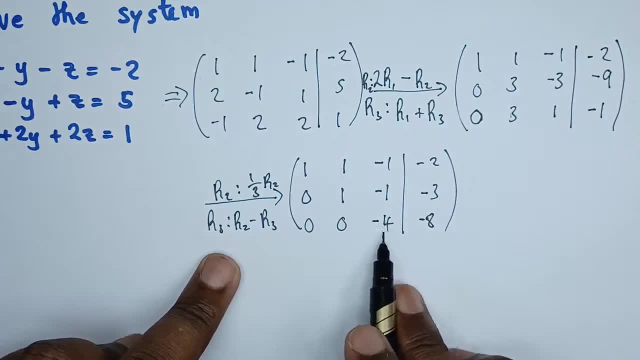 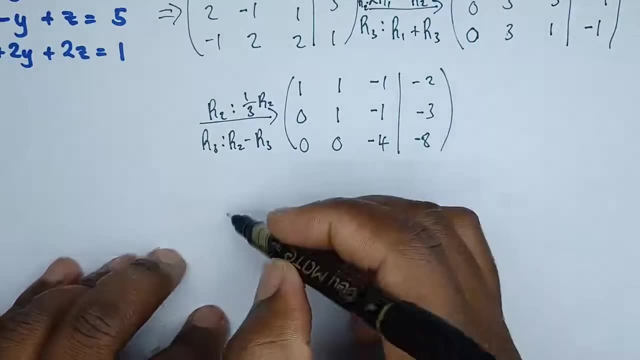 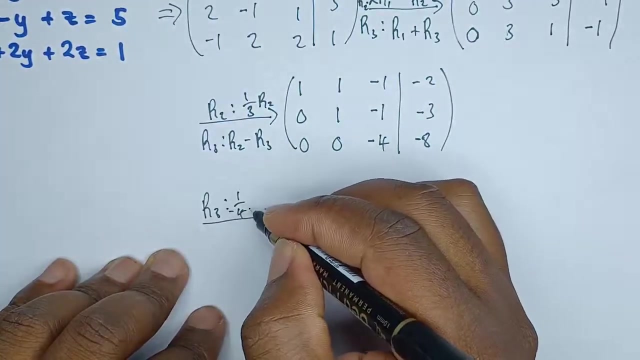 zeros. now we need a one there, one there and one there, so the only thing we're gonna meet is this part here. so how can you get a one here? very easy to get a one there. the operation we're going to carry out in row three will simply be one over four negative. we're multiplying everything in. 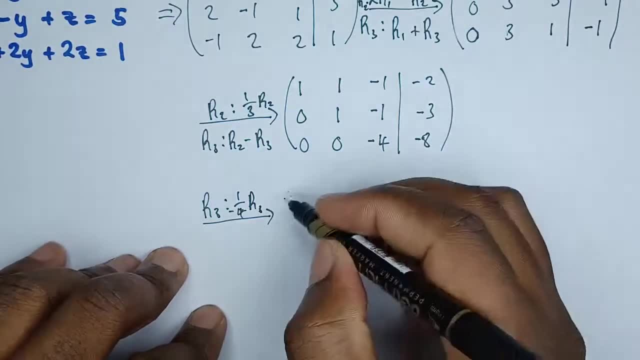 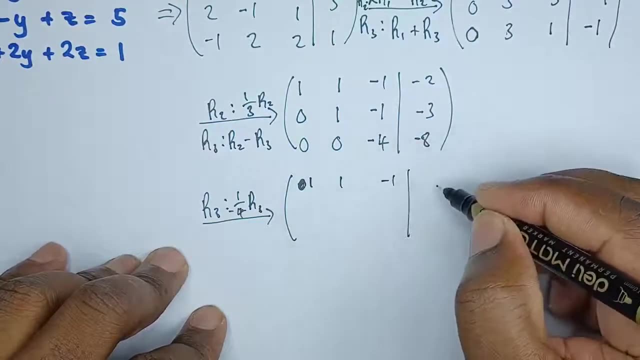 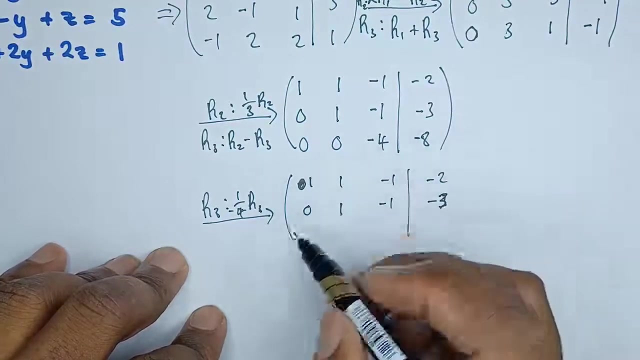 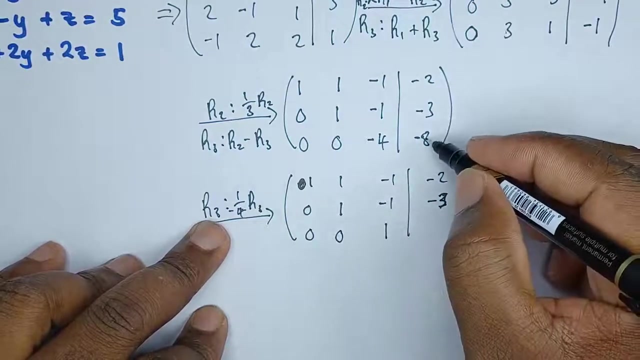 row three by one over four. so row one and row two will be maintained. uh, there's one there, sorry. one one negative one. negative two. zero one negative one negative three. so let's divide everything in row three by negative four. this will give us a zero. this will give us a zero. here we get a one negative eight divided by 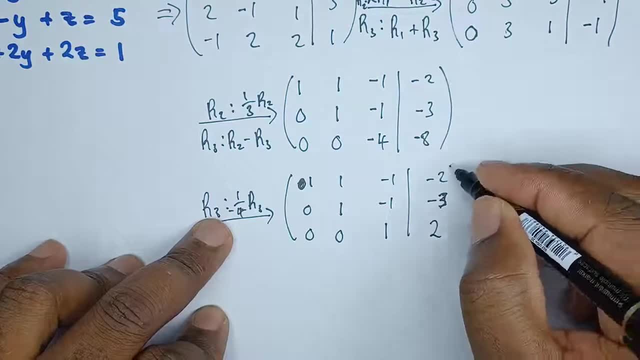 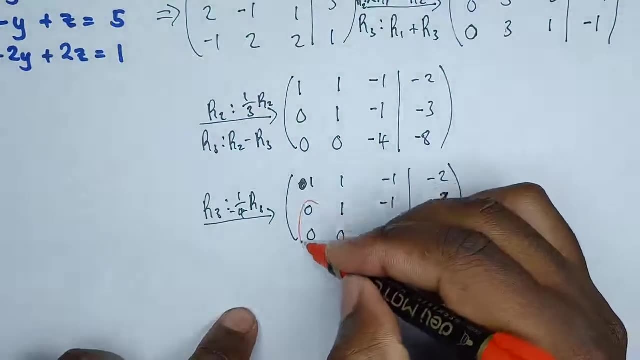 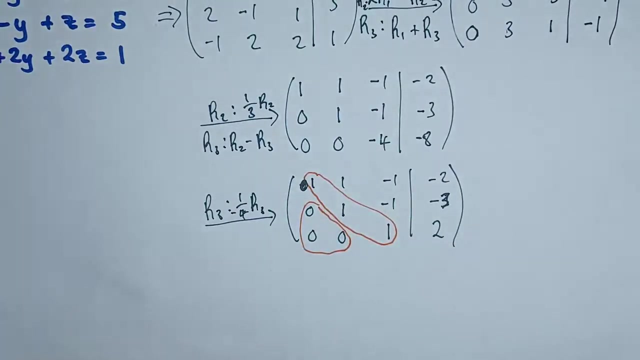 negative four, we simply get, uh, positive two. so this is what we have now. if you look at, um what we've done here, we've managed to achieve the three zeros here and the three ones there. whatever we have everywhere else doesn't matter. so now, this is what we're going to do. remember that this column 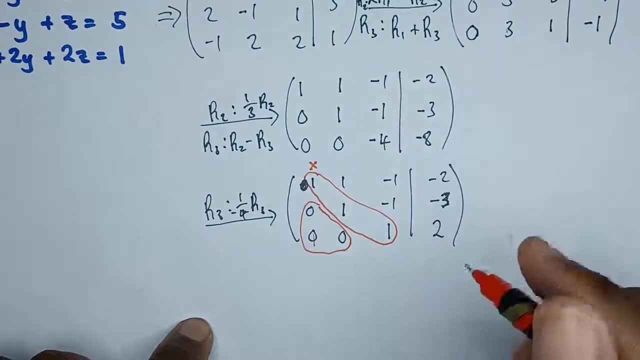 represents the x variables or coefficients. rather, this here represents the y coefficients, this here represents the z coefficients. so let's create, uh, three equations now here. so for the first one, what we're going to have will be one x, so that's just x plus one y, which is just y. 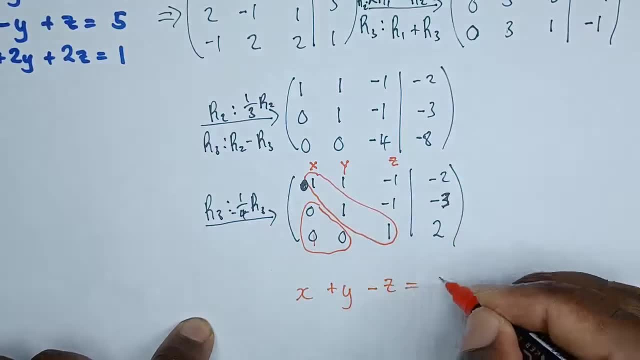 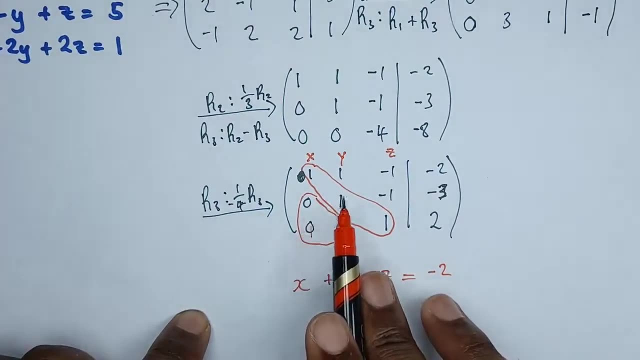 minus z. so minus z is equals to negative two. so that's the first equation. the next one: we're going to have the second row. we have zero, so we don't have x. we have one y, so that's just y. here we have minus z and everything is equals to negative three like that. then the last one: now we don't. 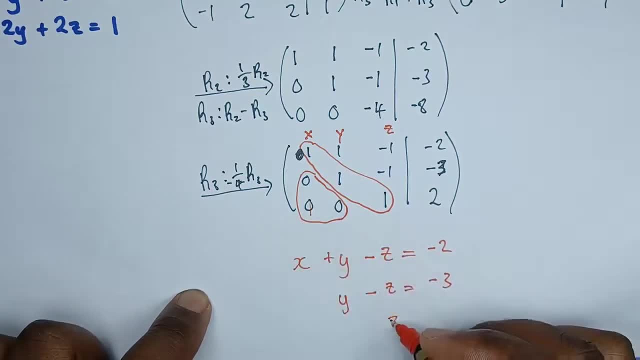 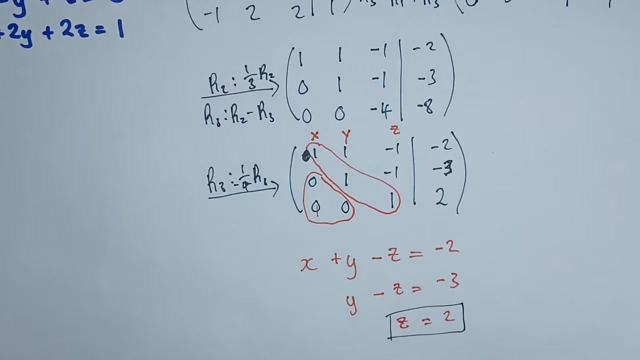 have x, we don't have y, we just have z. so z is equals to two. so just by observation, already we have found the value of z. so having found the value of z, let's go ahead and find out what we'll the value of Y. so to find the value of Y, we come back and use this equation and 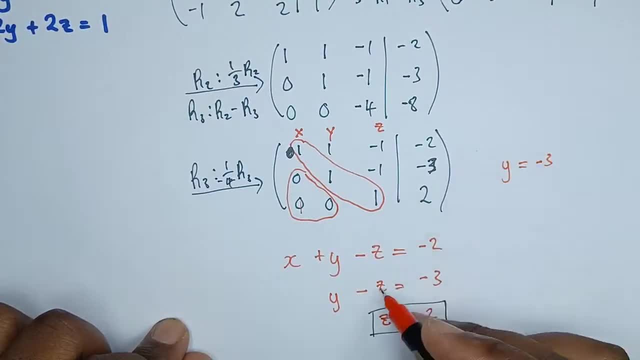 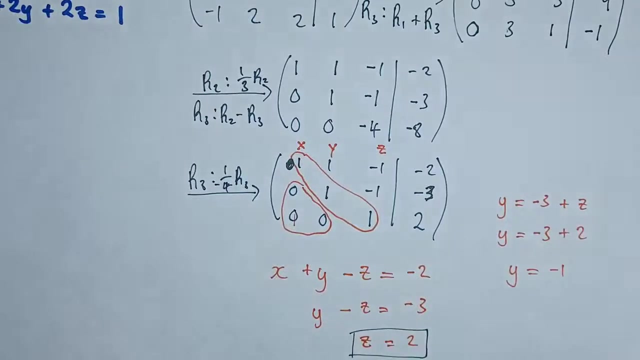 say Y is equals to negative 3. so let's push the Z to the other side, so it becomes a positive Z, so Y is equals to negative 3. remember, Z is 2 plus 2, so Y is equals to negative 1. so we have the value of Y. so, having found Y and Z, we 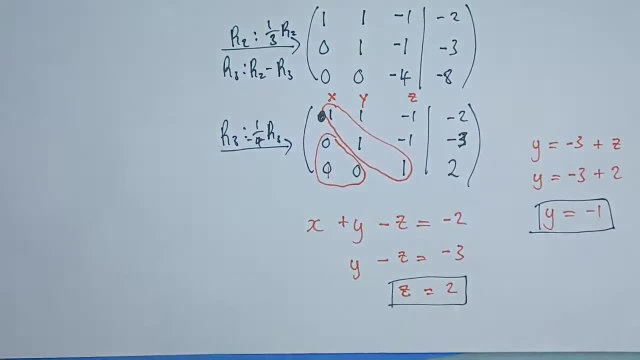 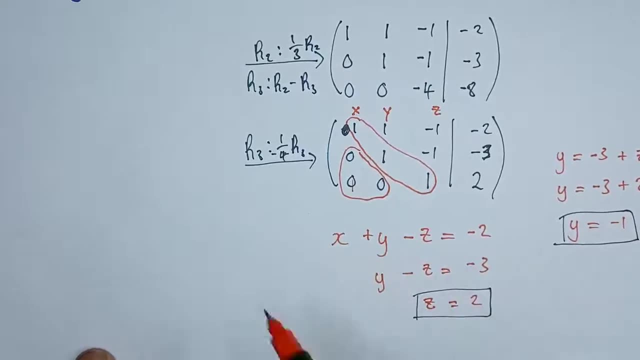 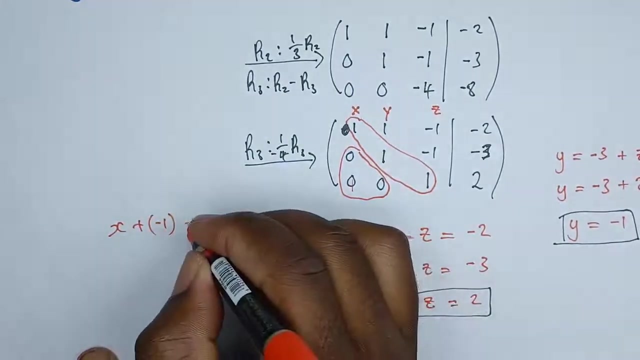 can now easily find the value of X. so this is what we're going to do again, just like we did for Y. we're going to use this equation: so X plus- remember our Y- is negative 1, so negative 1 minus Z- remember our Z is 2, so minus 2 is. 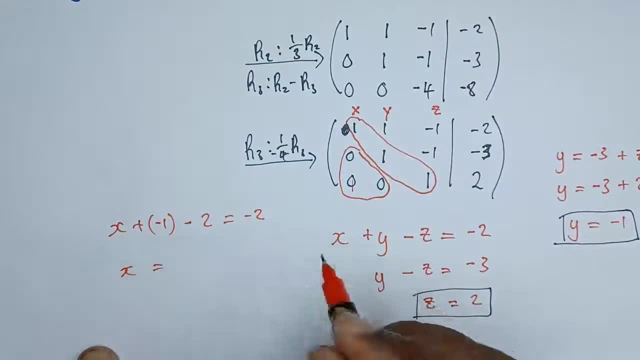 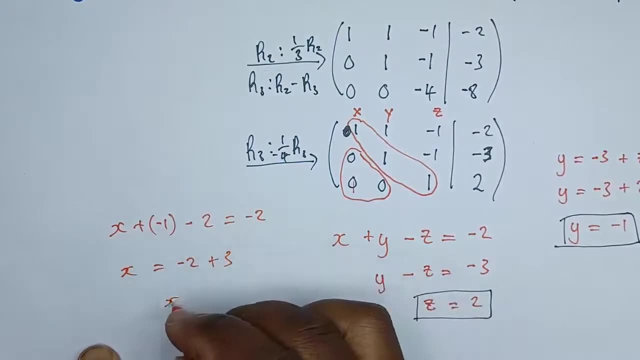 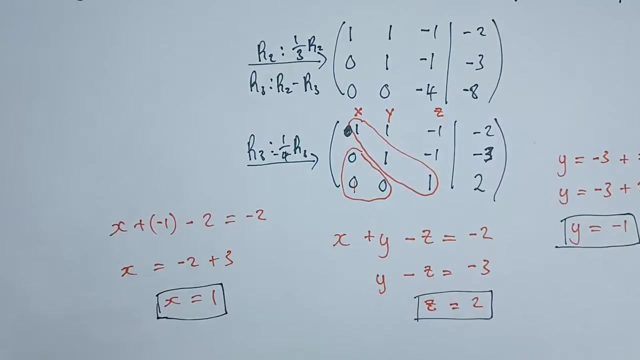 equals to negative 2. so X will be equals to negative 2, this one here negative 1. negative 2 is negative 3, closer side becomes positive 3, meaning that the value of x is equal to 1.. So this is the best way of solving this equation: by using the Gaussian elimination method. 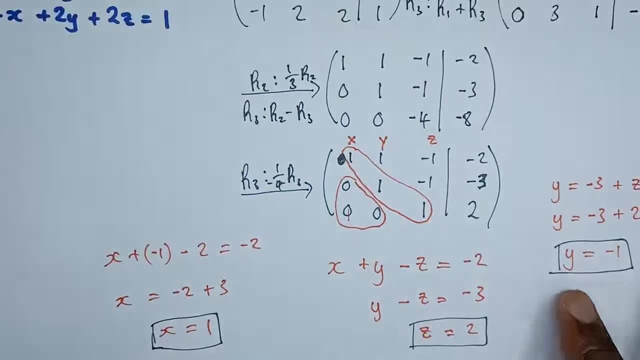 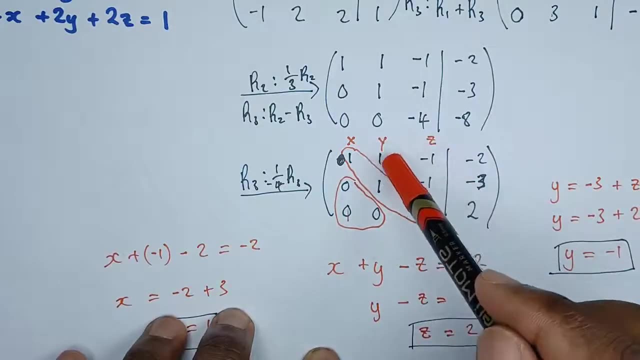 Okay, so now. one thing you need to know is that if you intend to proceed with this method here on these three positions, you can decide to put zeros here. If you put zeros here, what you're going to get are the three values for x, y, z here. 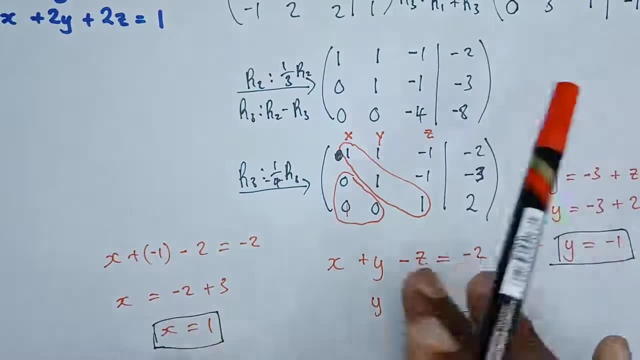 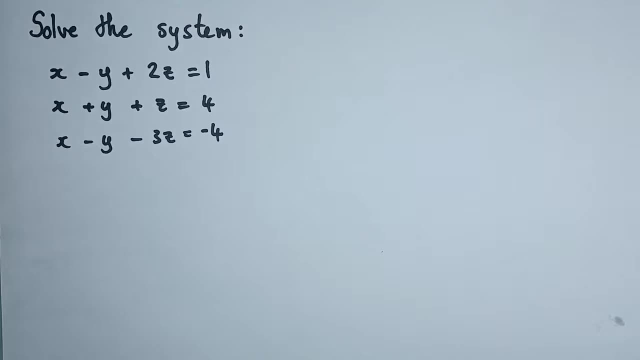 But even if you leave it here, you can just form these three equations and easily find the three variables. Okay, so I think we shall do this one instead, so that at least I don't waste much time. So the first thing we're going to do, like we did in the previous one, 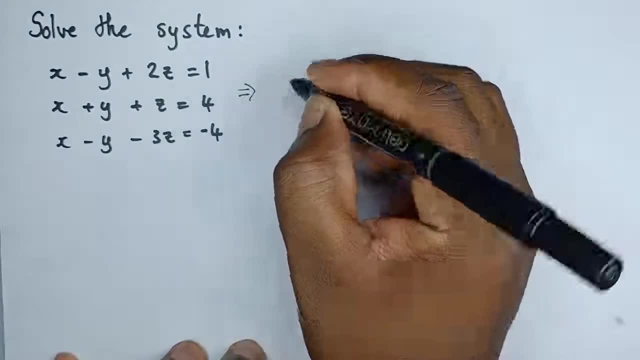 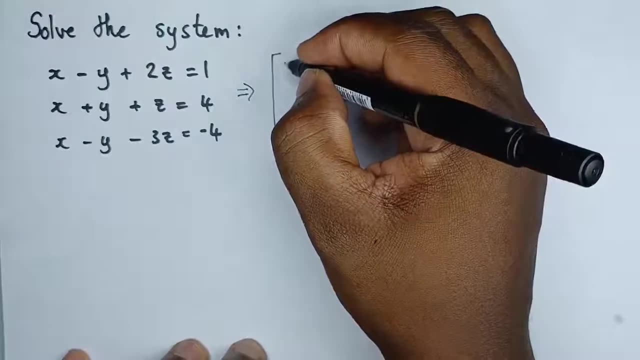 remember, we have to create something that looks like this: Coefficients of x: we have 1s throughout, So we have 1, 1, 1.. Coefficients of y: we have 1s throughout. We have negative 1, 1, negative 1.. 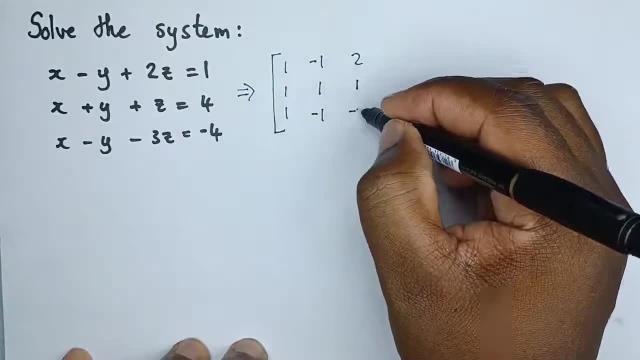 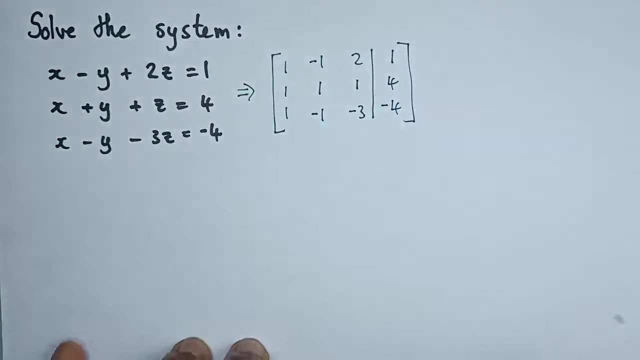 Coefficients for z. we have 2, 1, negative 3.. Then what we have there is simply 1, 4, negative 4.. Okay, so the first thing we're going to do is we need 1 here, remember. 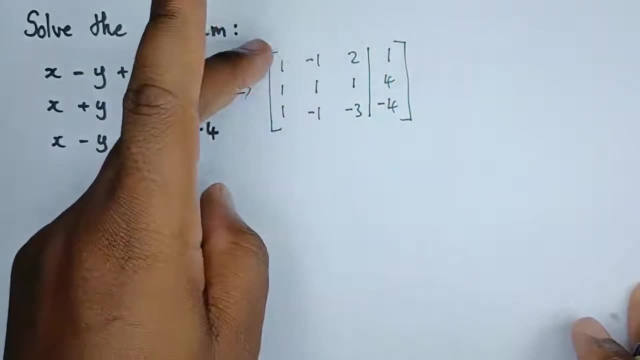 But before 1, it's always easier to start with zeros. So for 1,, we're okay, because we already have a 1 there. we need a 0 here. So to get a 0 here, it's very easy. 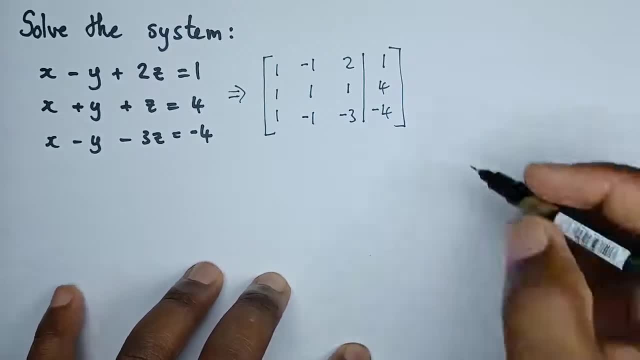 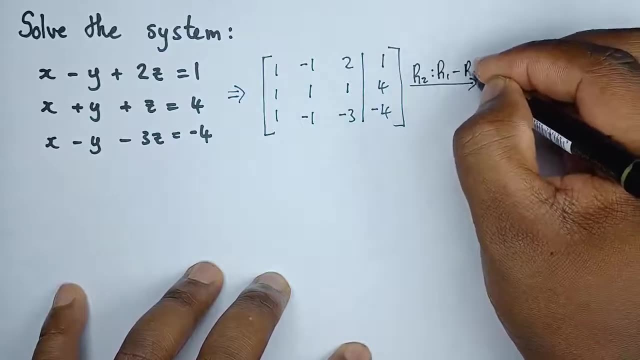 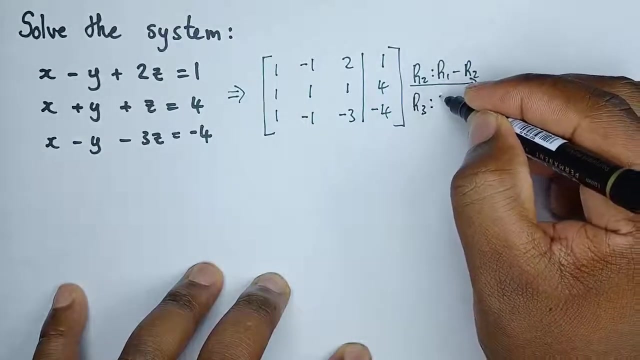 because you just use 1.. 1 and 1 to cancel themselves by simply subtracting. So the operation in row 2 will simply be row 1 minus row 2.. We subtract, they cancel. The operation here in row 3 will simply be row 1 minus row 3.. 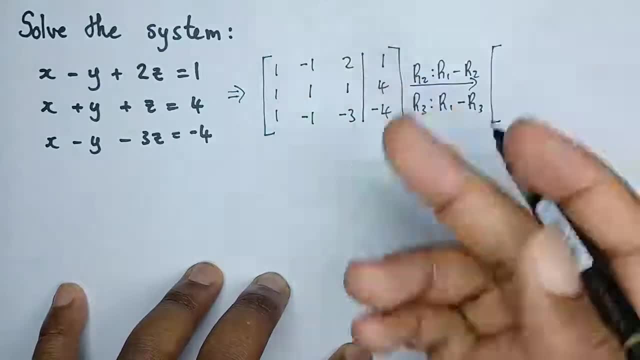 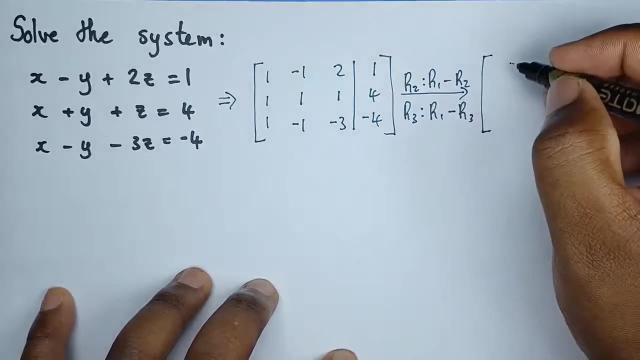 We subtract, they cancel. same thing. It doesn't matter if you use row 2 as well. we still get to the same required answer. So row 1, we haven't tampered with it, but it's okay. Negative 1, 2, 1, that's row 1.. 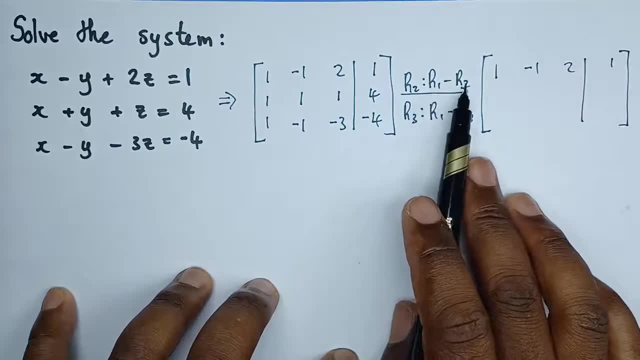 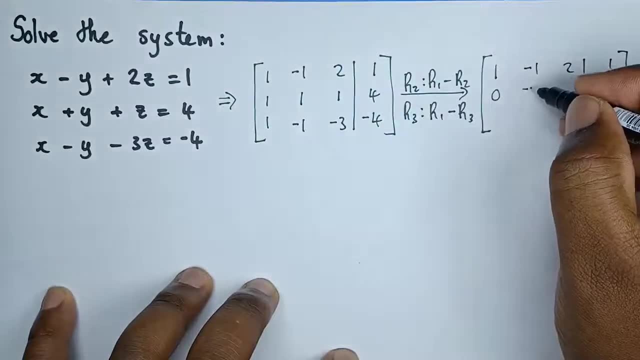 Row 2, we're subtracting row 1 minus row 2.. The operation is on row 2.. So 1 minus 1, 0.. Negative 1 minus 1, negative 2.. 2 minus 1, that's 1.. 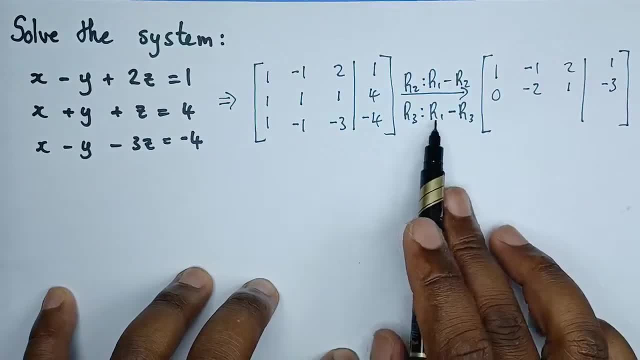 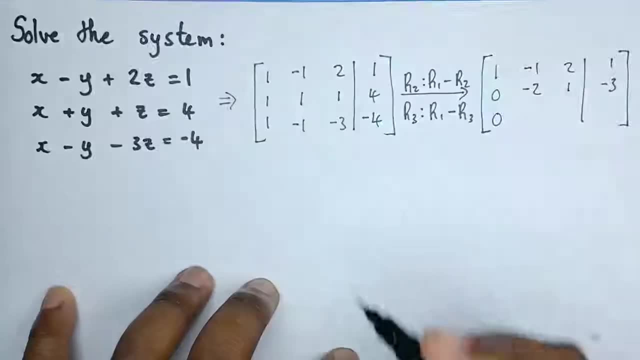 1 minus 4, that's negative 3.. Then 1 minus 3, now Row 1 minus row 3, the operation is on row 3.. So 1 minus 1, 0.. Negative 1 minus negative 1, we'll get a 0.. 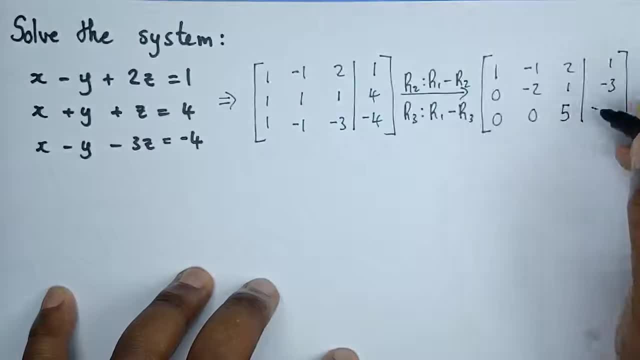 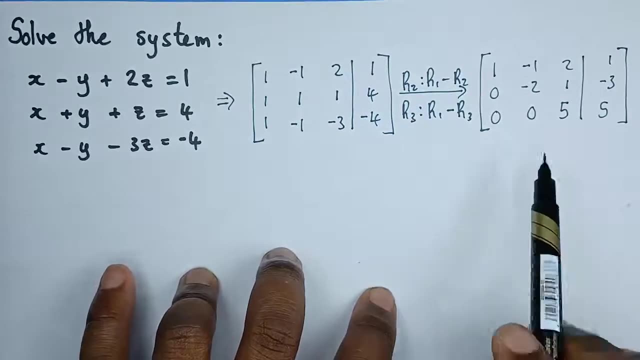 2 minus negative 3, we'll get a positive 5.. Then 1 minus negative 4, we'll get a positive 5 as well. Okay, so, if you've seen, we've achieved the three 0s that we wanted. 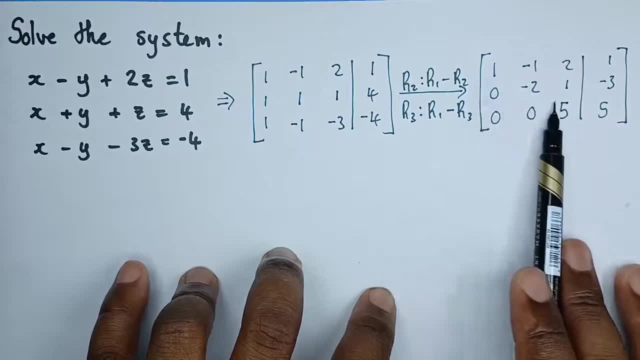 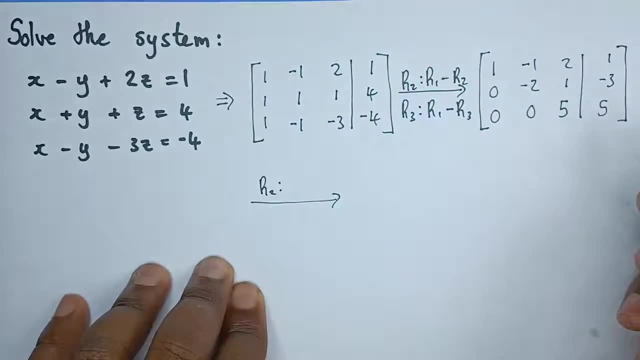 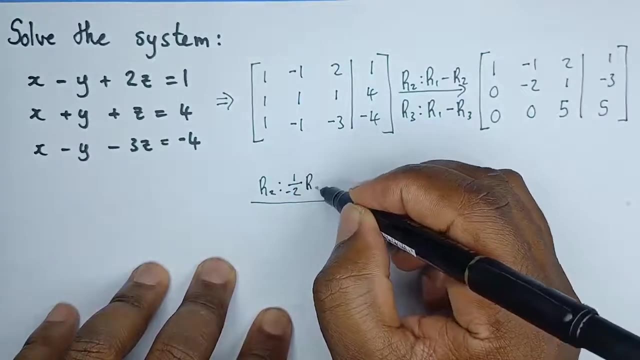 The only thing we need are the 1s in this diagonal To get a 1 here. it's very easy. So, row 2, the operation is just multiply by the reciprocal, which is row 2.. So like that On row 2, just multiply by the reciprocal, which is negative 1.. 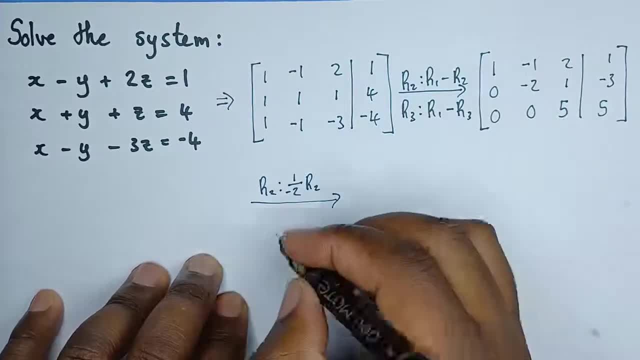 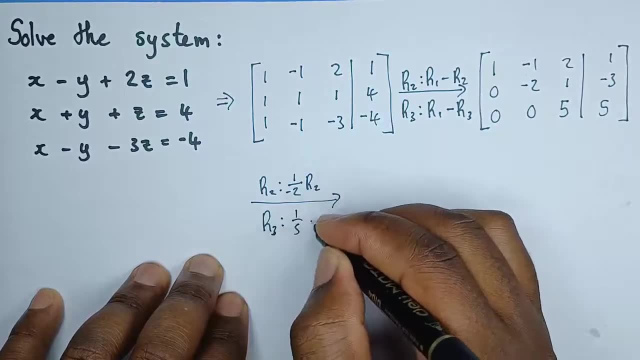 Then in row 3, again, multiply by the reciprocal, So row 3, the reciprocal of 5. Since we need a 1 there, it's simply 1 over 5.. So that's on row 3.. So row 1, not touched. 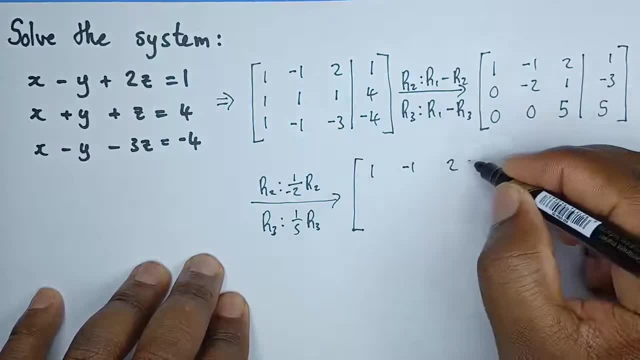 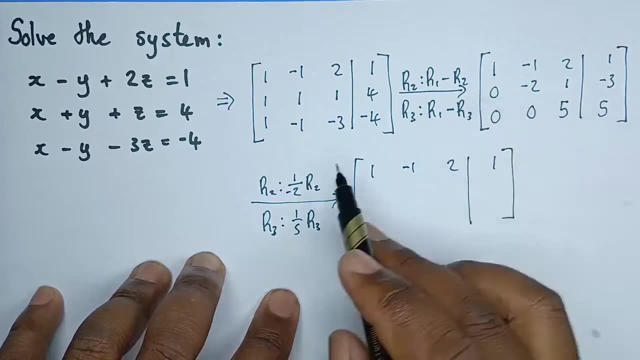 So we'll remain as it is, Negative 1 there. There we have the 2.. There we have the 1.. Here, remember, we're multiplying everything by a negative half, or dividing everything by negative 2.. So we get a 0 here. we get a 1 here. 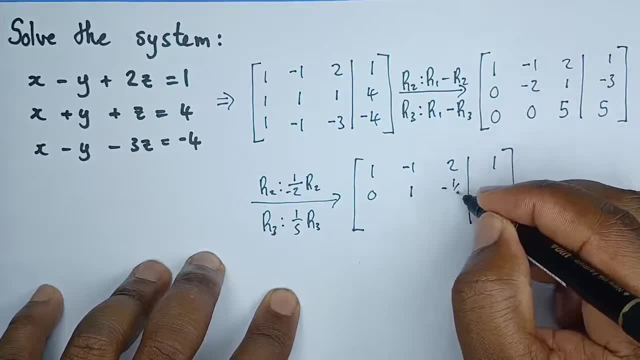 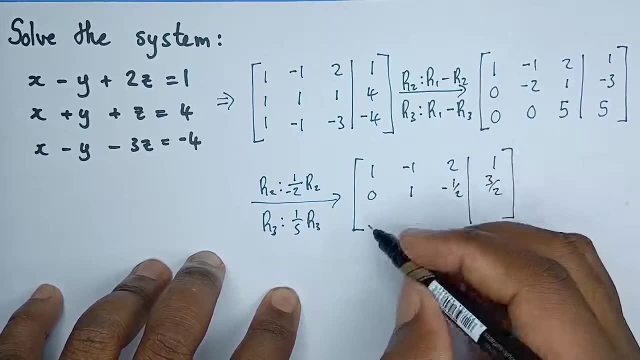 Divided by negative 2, we get negative half. Divided by negative 2, we get 3 over 2.. So row 3, we're dividing everything by 5.. So 0, 0, there 1, there 1.. 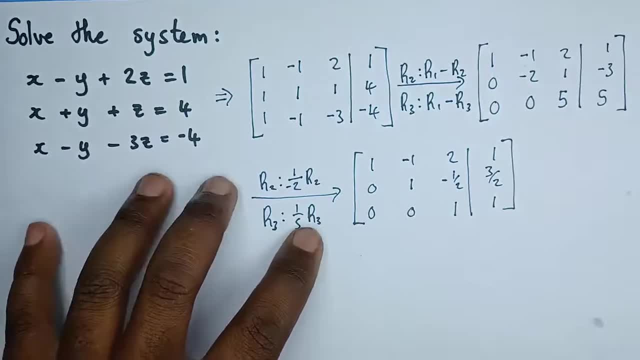 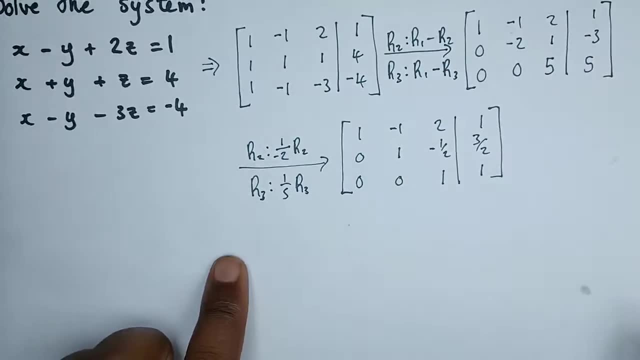 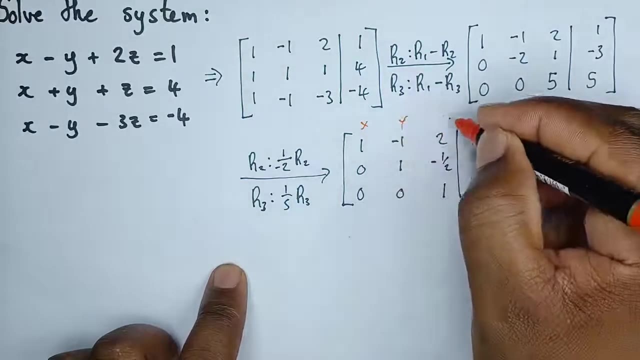 Okay, So now let's create the three equations that we did in the previous example. So the three equations. I'll just start with the simplest ones, which is the third one: x is 0, y is 0.. Remember, this is x, this is y, this is z. 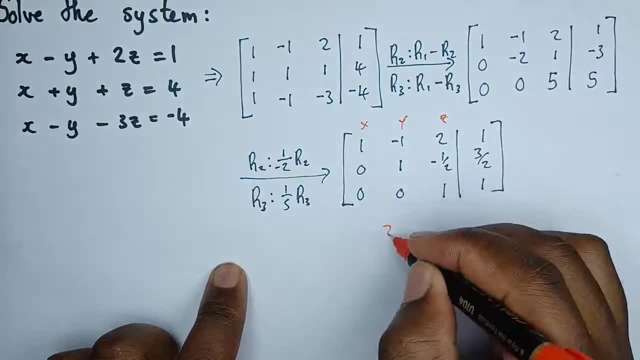 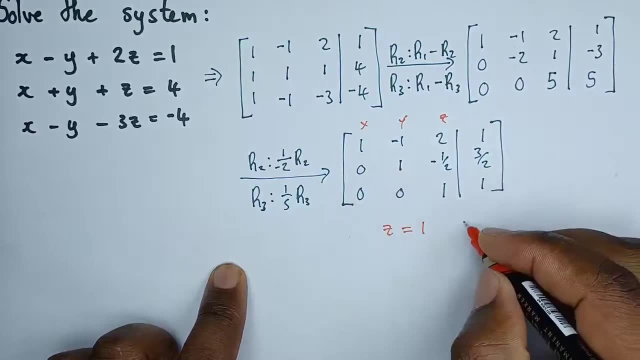 x is 0, y is 0, z is 1.. So z is simply equals to 1.. We're done. In the next one we know that x is 0 but y is 1.. So y minus half z. 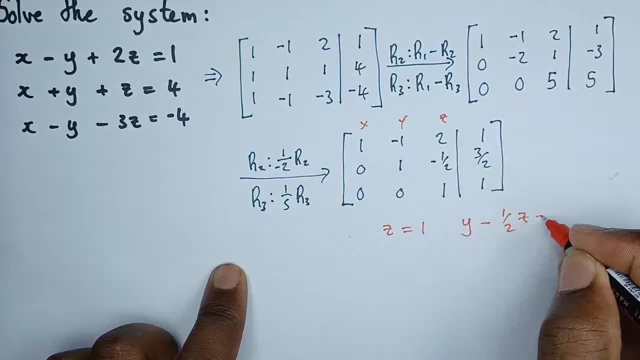 So minus half z, Everything is equals to 3 over 2.. But we know what z is. z is 1.. So y minus half times 1, there is equals to 3 over 2. So y is equals to 3 over 2.. 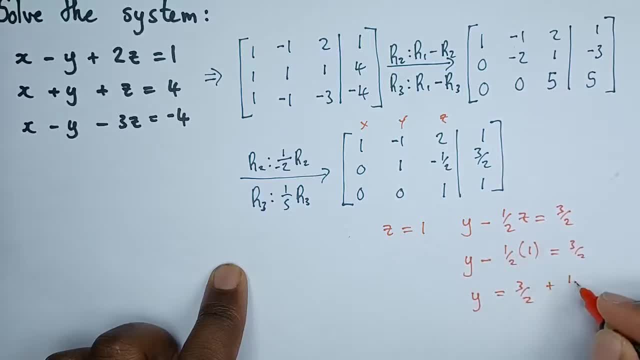 This negative half can go to the other side to become a positive half, Like that. So 1 over 3, or rather 3 over 2 plus 1 over 2.. That's just 1 and a half z. That's just 1 and a half plus half. 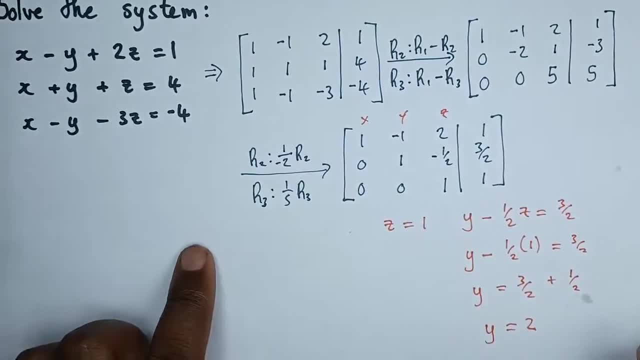 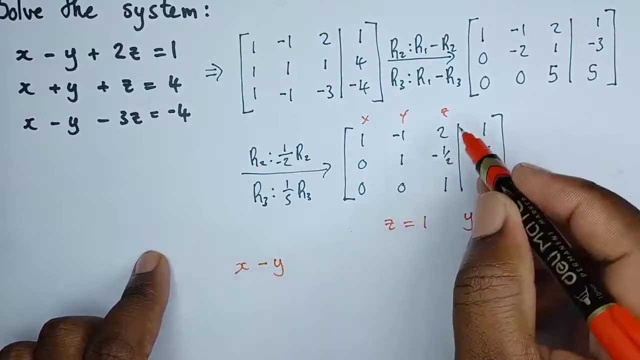 We simply get a 2. We have y, We have z. We can easily find x by saying: x, there is 1., y, there is negative z, there is a 2. So plus 2z, Everything is equals to 1.. 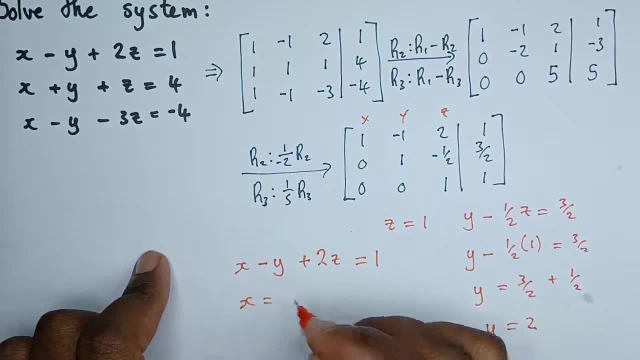 So we're finding the value of x. Let's make x a subject, So x will be equals to 1 plus y minus 2z, Because both of them go to the other side. So x will be 1 plus what is y. 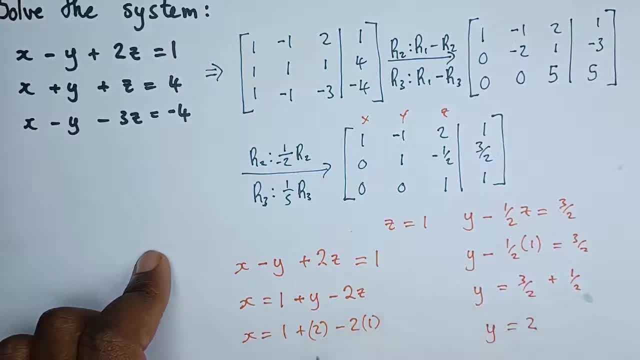 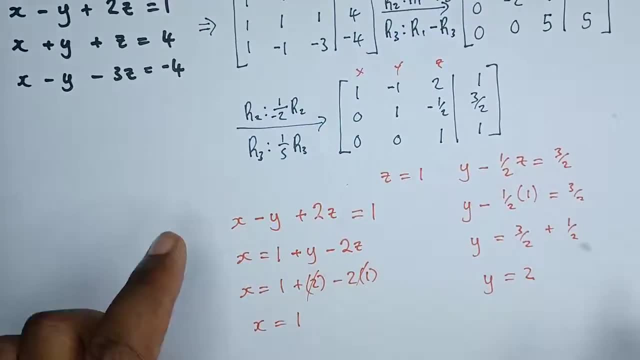 2. Minus 2.. What is z: 1.. So x will be equals to these two. cancel, because 1 is positive, 1 is negative. So the value of x is simply equals to 1.. So there we have it. 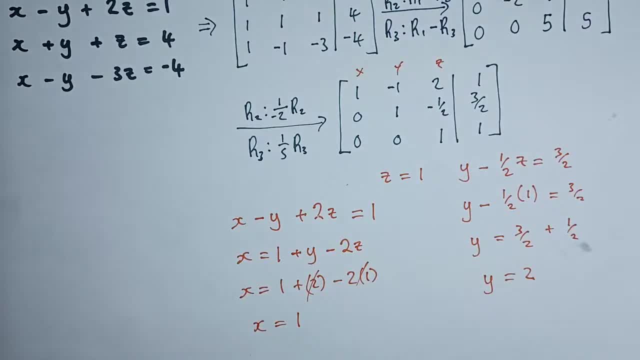 That's how we solve a 3 by 3 system: by using the Gaussian elimination method. Please understand that even if you have a 4 by 4, make sure to make the major diagonal to have 1s and everything below it to have 0s. Then you can just use the same procedure. Thank you very much. 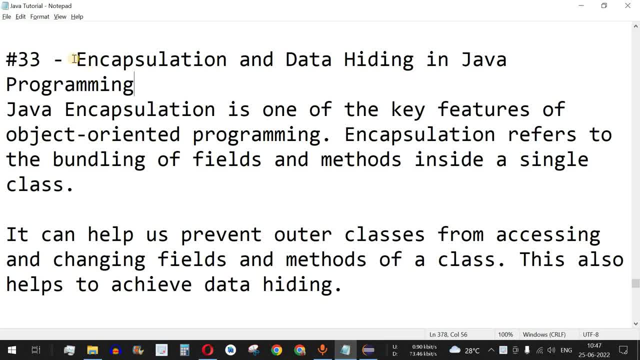 hey, what's up, guys? welcome to another video in which we are going to learn about encapsulation and data hiding in java programming. so, guys, java encapsulation is one of the key features of object oriented programming. so, as we had seen previously, we can implement java encapsulation.